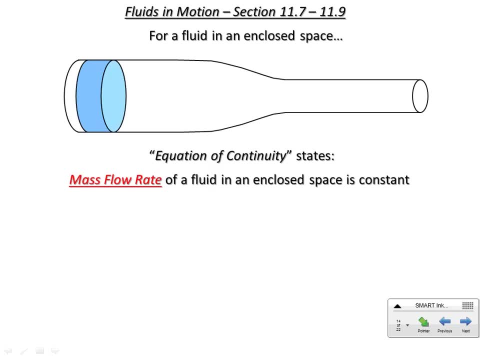 a certain. you know, in this volume there's a certain amount of fluid. in an enclosed space There's a certain mass of fluid, depending, of course, on the fluid's density. All right, What that says is really, we can say that mass per unit time. let's call this an area. 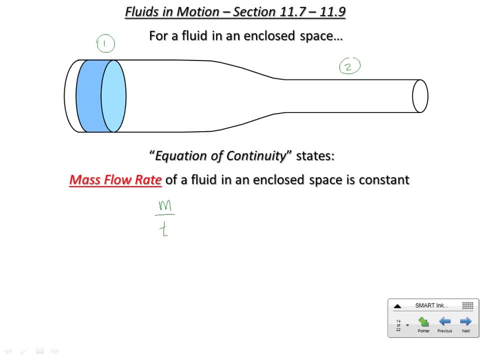 one and mass per unit time in area two have to be the same thing. The same amount of mass basically gets to a point and leaves a point in the same amount of time, no matter what's true about the enclosure itself. Okay, So we can write this as mass. we can write as: 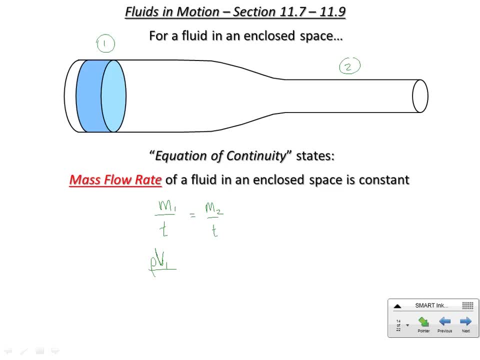 rho V1 volume right over T equals rho V2 over T. Now again, we are assuming the gas is incompressible. incompressible meaning the density doesn't change. All right, So if density is the same everywhere, well we. 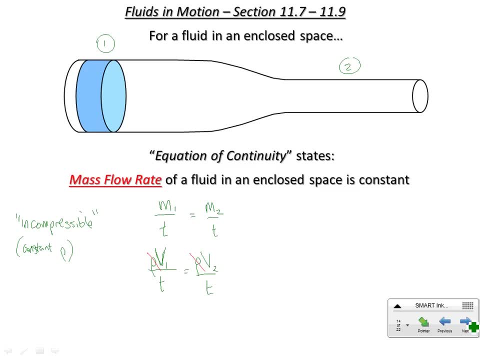 say: that's true, Okay, And we call this. where this is mass flow rate, we call this. if it's volume per unit time, we call it volumetric flow rate. Oops, So we're saying that volumetric flow rate has to be constant, And that might be. you know, the density doesn't change. 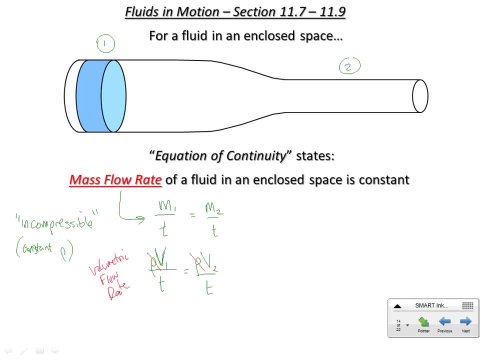 I don't know Easier to or as easy to understand as the mass flow rate thing. This you know. this says that if a gallon of water per minute comes into a point, then a gallon per minute must leave that point. Sure, Because of where the other fluid go. Okay, Now we can take. 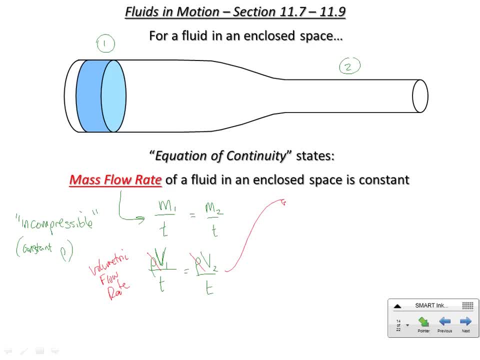 this into well. let's see the volume of this subsection of fluid. we would say this has area A And let's call this, like I don't know, a delta X, All right, So we can say that volume. 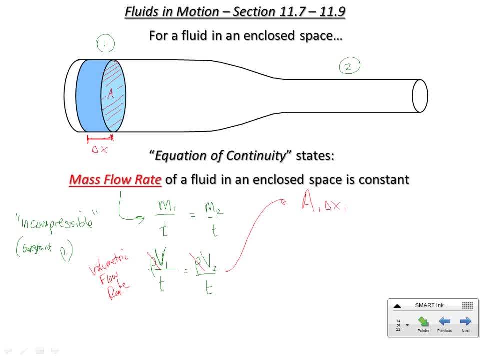 is really A1 delta X1 over T. Well, that's got to be equal to A2 delta X2 over T. Well, over here in area 2, what's that volume of fluid It's going to look like? well, since the area gets so much smaller, right, it means. 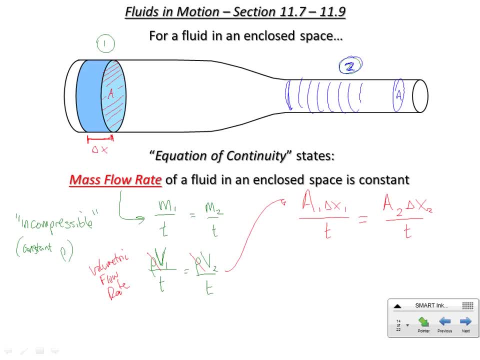 that our delta X has to get a lot bigger. Okay, And what you can also tell is if this delta X has to be a lot bigger in the same amount of time. what we're really saying is that there is this relationship: A1, V1 is A2, V2, right. 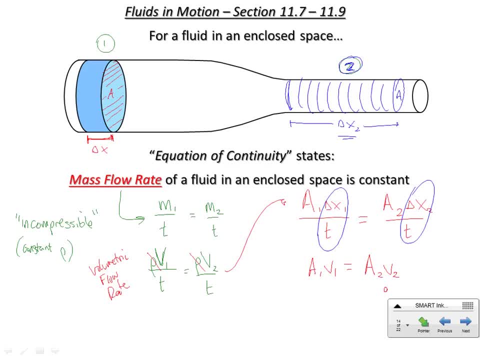 And so we can see that there is this relationship. And, in my case, if I set this to the same amount of fluid past a point per unit time, well, if the area of that enclosure gets smaller, it means that the fluid has to speed up. Okay, This is what we call the equation of continuity. 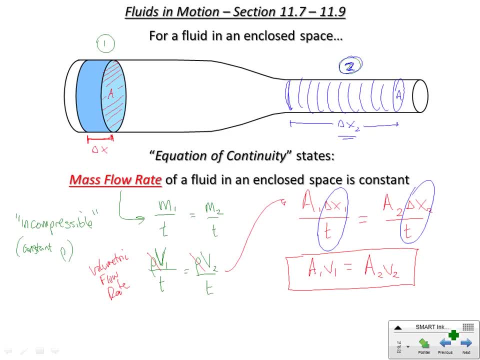 We also just define. here's yet another place where we're repeating some. repeating a variable We call Q is our, what we call volumetric flow rate, which you can call volume of traffic. So we can just define, let's say, volume of air in the past per minute compared to. 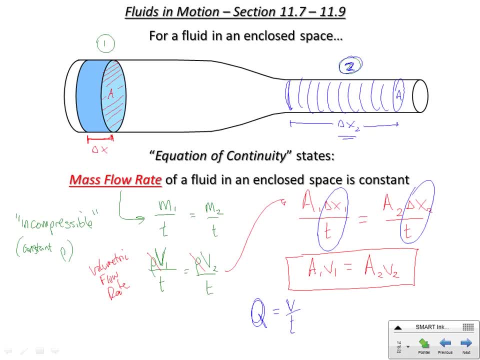 the volume of air in the past We can also just define. here's yet another place where we're repeating. a variable We call Q is our what we call volumetric flow rate, which you can call volume of air, sea Well, volume, all right, I've got to be careful in a second here. 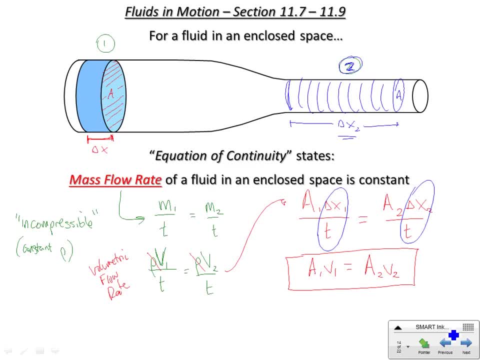 We'll be back up Now. this delta x over t is velocity. right, These are velocities, very important, Velocity velocity. all right, Notice, small v, not volume. okay, When we talk about this over here, this v is volume okay. 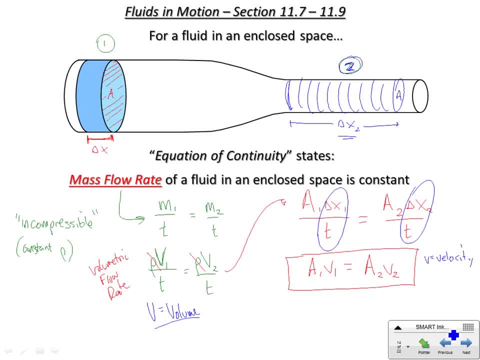 So we just want to make sure that we define this one quantity that we call q, which is our volumetric flow rate. So it's v big V. we'll do like this. so it's like a capital V over t, also equal to a times v. 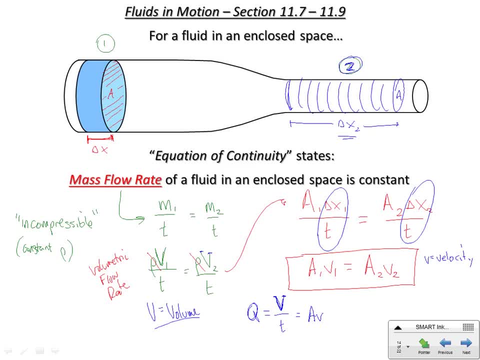 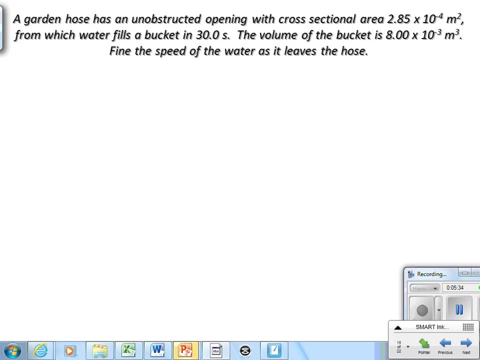 All right. so two ways of finding volumetric flow rate, either volume per unit time or area times. volume, Sorry, area times, velocity, All right. so here's a sample problem with this continuity sort of concept. and it says: we have this garden hose, blah, blah, blah. 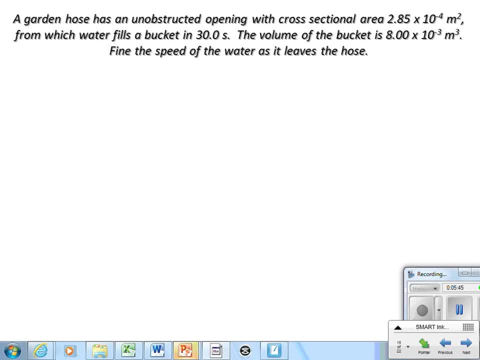 the cross-sectional area is that from which water fills a bucket in 30 seconds. the volume of the bucket is that: find the speed of the water. Okay, so let's see To find this, find, find, find the speed of the water as it leaves the hose. 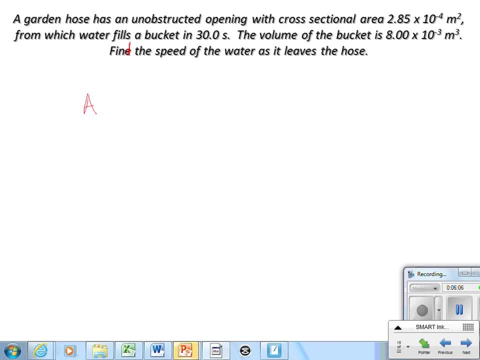 So if we're going to find speed of water, it's really going to be part. you know it's going to be this a times v. So for the hose we can use a times v. Well, continuity could say. 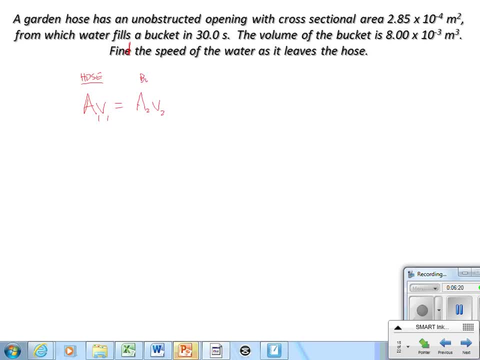 A2V2 bucket right, except we don't know the area of the bucket or the well. the water doesn't flow through the bucket so it'll be hard to define a velocity there. but what we do know for the bucket is volume of the bucket. 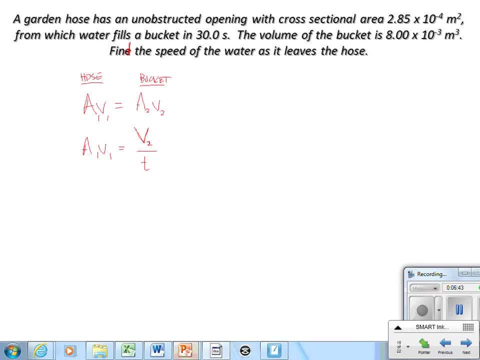 and how long it takes, okay. So how about I do this? We'll call this hose hose and we'll call this bucket bucket, bucket. okay, So if we want to find the speed of the water in the hose, we do this. 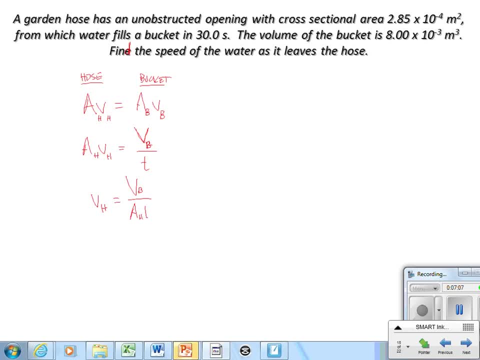 v bucket over area hose times the time. all right, That's. the volume of the bucket is 8. It's 10 to the negative. third cubic meters over. let's see area area. Oh yeah, it gives us area which is nice, 2.85 times 10. 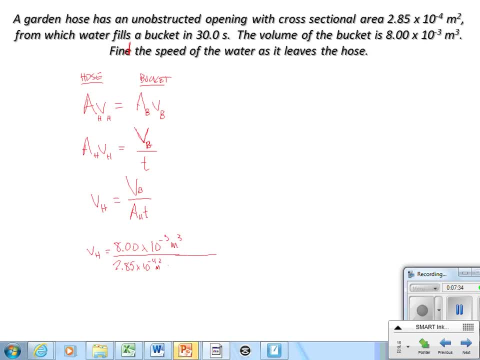